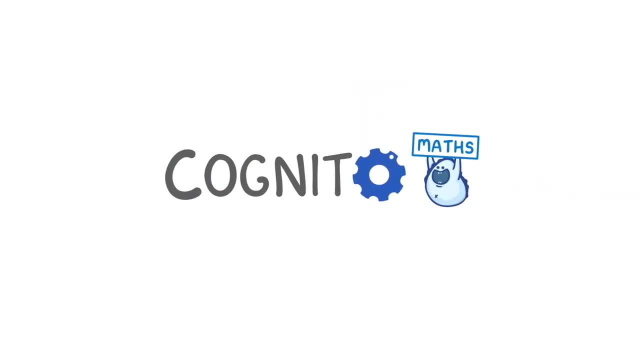 In this video, we're looking at how to find the volumes of both spheres, which are tennis ball or football shapes, and hemispheres, which are basically spheres that have been cut in half. To find the volume of a sphere, we use the 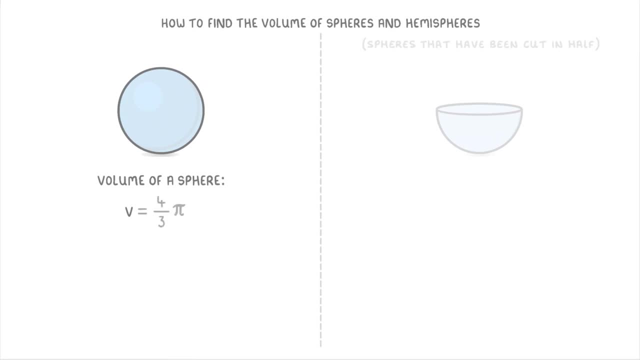 formula: volume equals four-thirds pi r cubed, where r is the radius of the sphere. So if our sphere had a radius of 5 cm, then its volume would be four-thirds times pi times 5 cubed, which would give us 524 cubic cm. Now, because a hemisphere is just half a sphere, 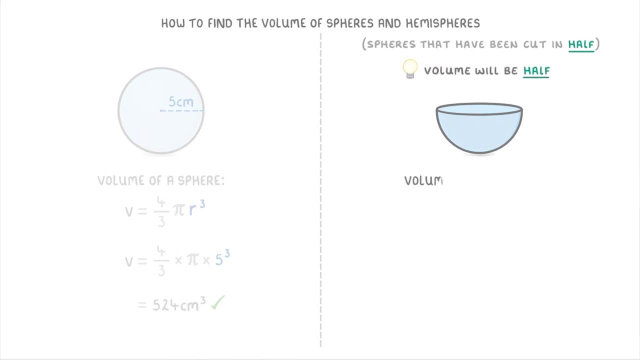 its volume will be half the volume for the entire sphere, which would give us just 6 cubic cm. Now, because a hemisphere is just half a sphere, its volume would be half the half as well. So to calculate the volume of a hemisphere, we can just use the sphere formula. 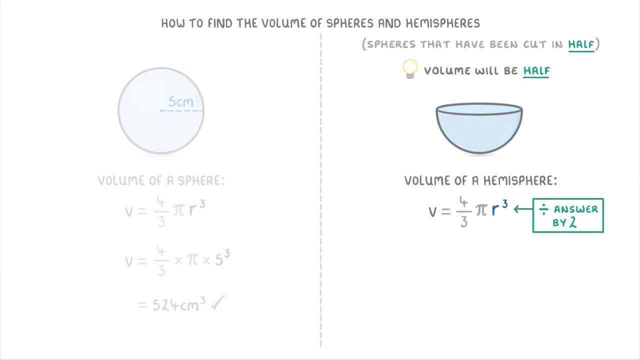 that we used before and then divide our answer by 2.. So if the radius was 5 centimeters again, then we'd still do- volume equals 4 thirds times pi times 5 cubed to get 524 cubic centimeters. but then we'd have to divide the answer by 2 to get a volume of 262 cubic centimeters for our. 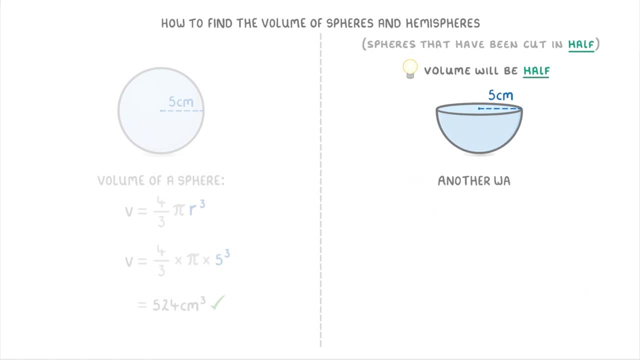 hemisphere. Another way to work out the volume of a hemisphere, though, is to use its own formula of volume equals 2 thirds pi r cubed, and you might notice that this is exactly the same as the volume for a sphere, except it has a 2 here instead of a 4.. So, basically, because we've halved. 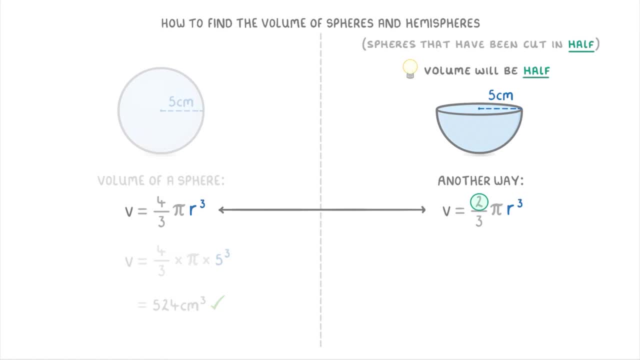 the 4 to a 2, the overall volume will be half as big as well. So it gives us the volume of a hemisphere rather than a whole sphere. And to show you that it works for this hemisphere we're to do 2 thirds times pi times 5 cubed. 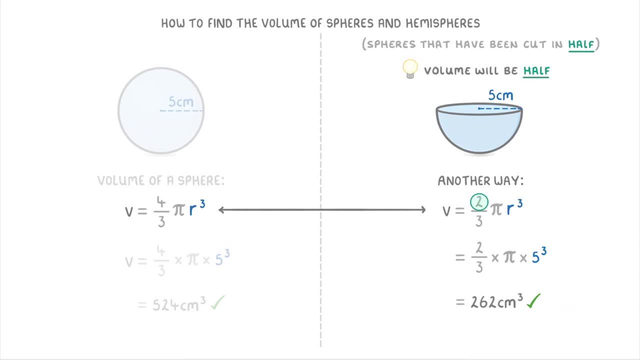 which would give us 262 centimeters cubed, which is exactly the same as we got before. So the takeaway here is that it's completely up to you whether you want to use the sphere formula and then half your answer or use the hemisphere formula. Either way, you're going to end up with